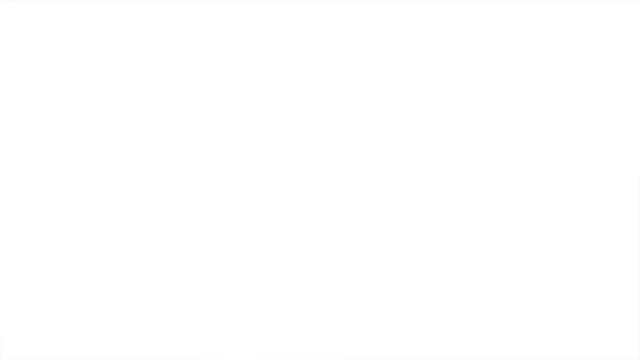 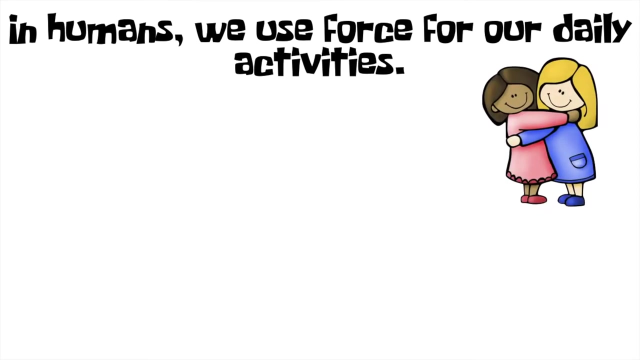 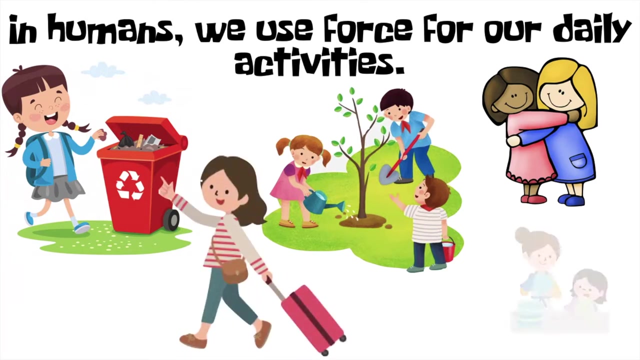 In humans, we use force for our daily activities, For example, hugging your friend, throwing your garbage, doing some chores, pulling your bag and even helping your mom washing the dishes. These are some examples of daily activities that we use force. 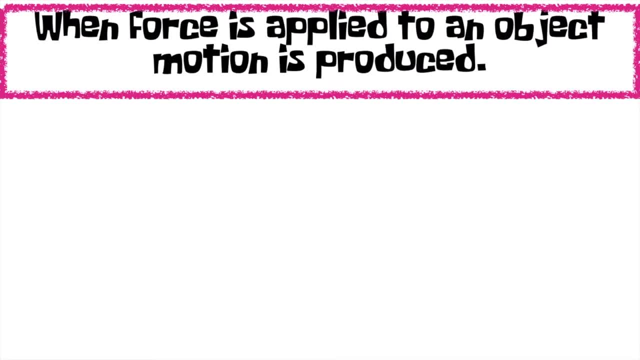 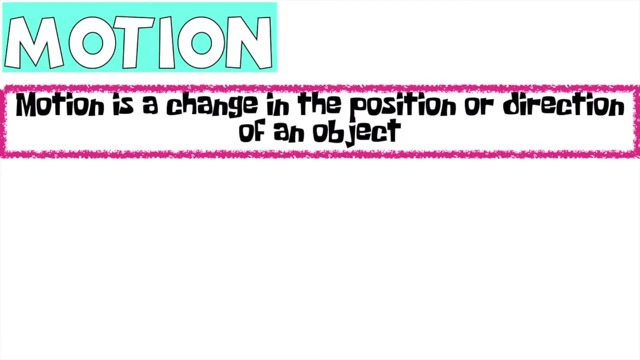 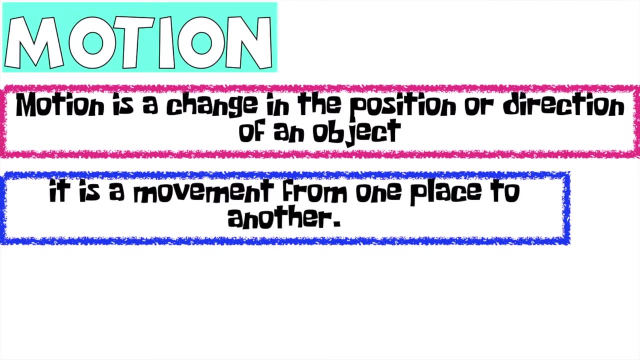 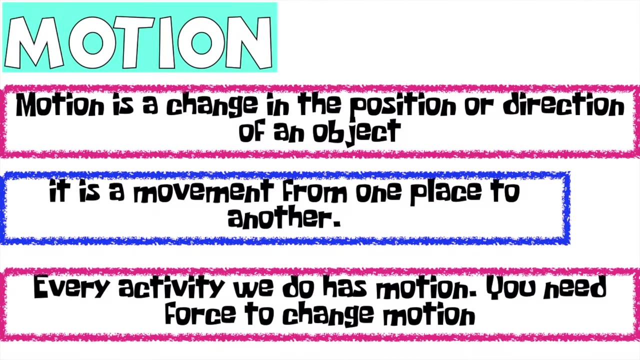 When force is applied to an object, motion is produced. When we say motion, it is a change in the position or direction of an object. It is a movement from one place to another, And also every activity we do has motion. You need force to change motion. 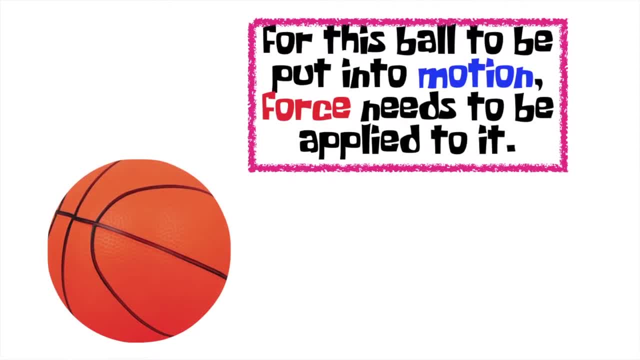 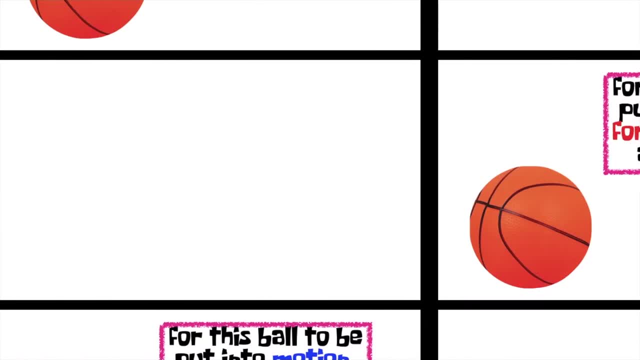 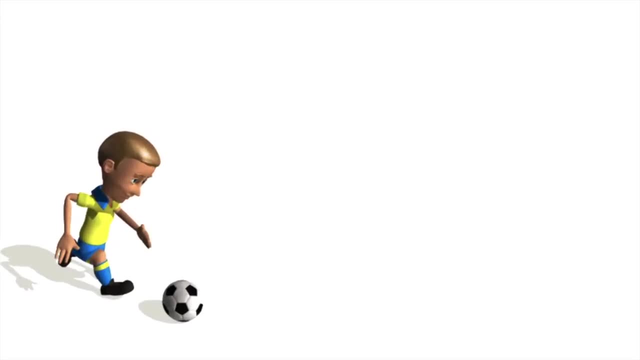 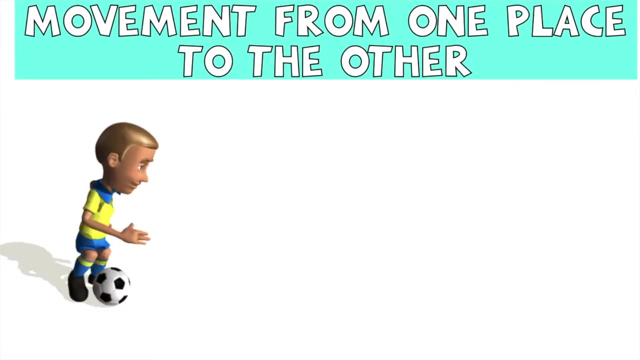 For this ball to be put in motion, force needs to be applied to it, Just like this. Let's see how motion occurs. Are you ready? Let's have the first example. Look at the boy kicking the ball. The motion occurs here is movement from one place to the other. 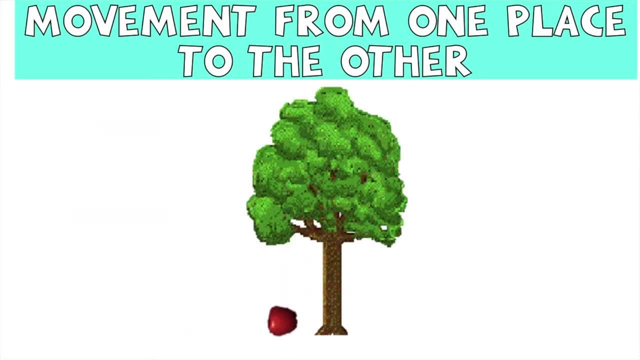 Let's have another example. Look at the boy kicking the ball. And also every activity we do has motion. And also every activity we do has motion. An apple fell on the ground. This is a movement from one place to the other. 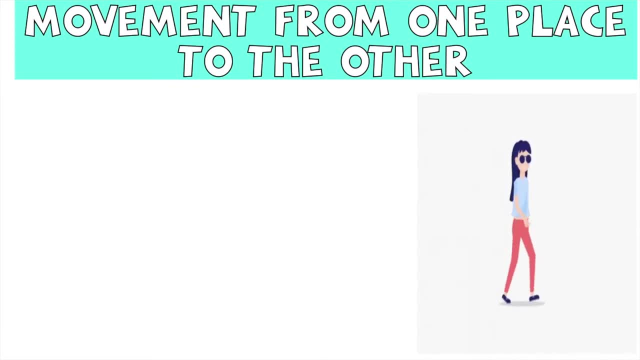 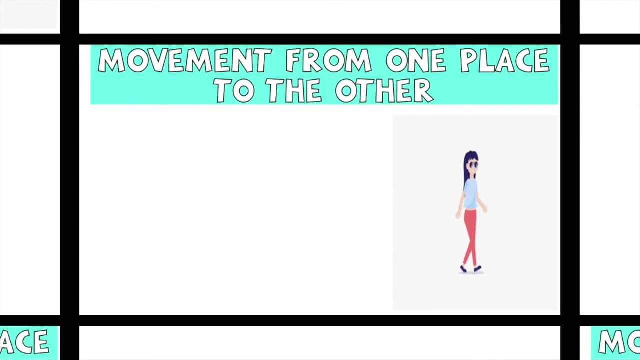 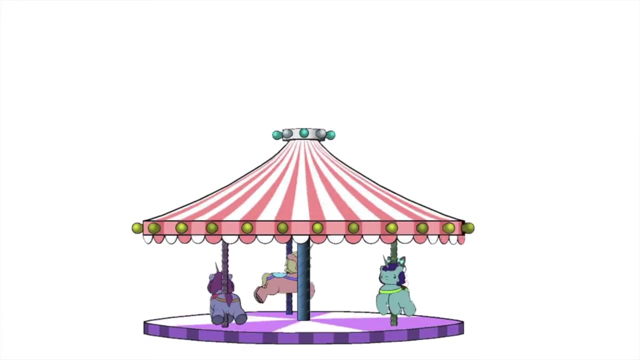 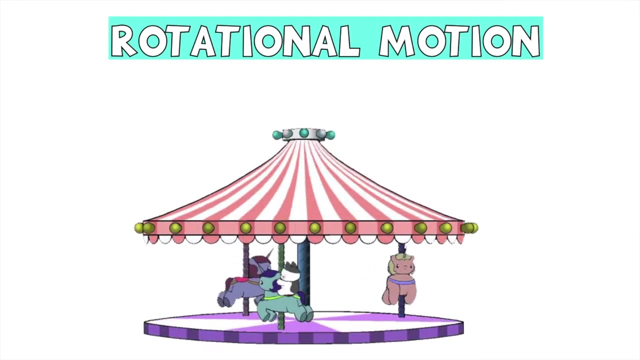 Next walking. The motion occurs here is movement from one place to the other. How about if we have this? As you can see, the movement of this one is in circular mode. So the motion occurs here is rotational motion. Let's have another example. 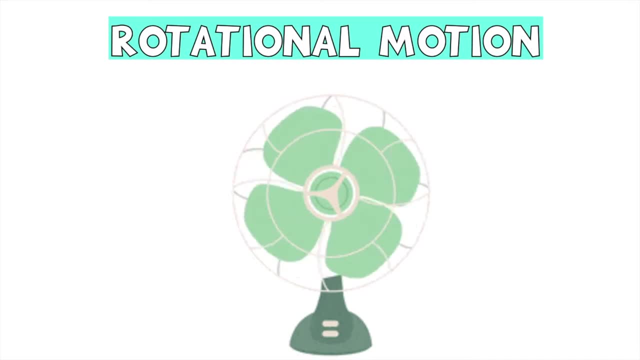 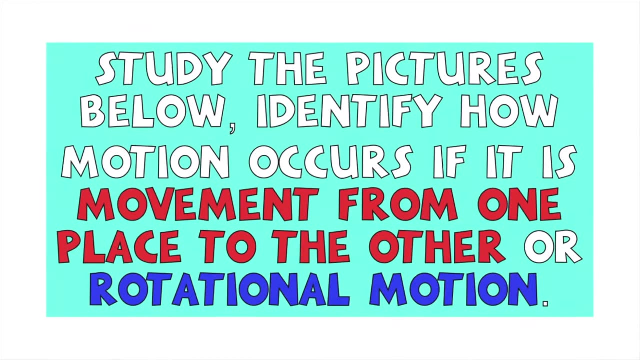 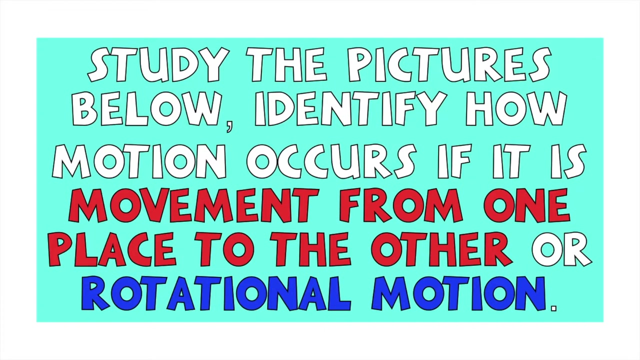 Again, this is an example of rotational motion. The movement is in circular mode. So now let's study the pictures below And identify how motion occurs, if it is movement from one place to the other, or rotational motion. Are you ready? Let's have this. 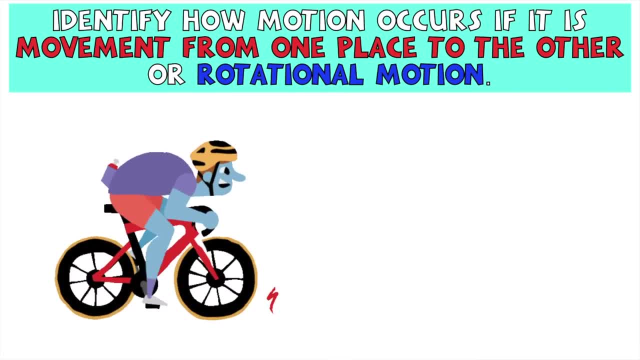 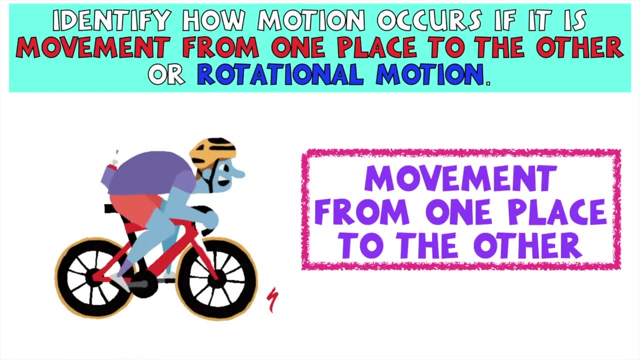 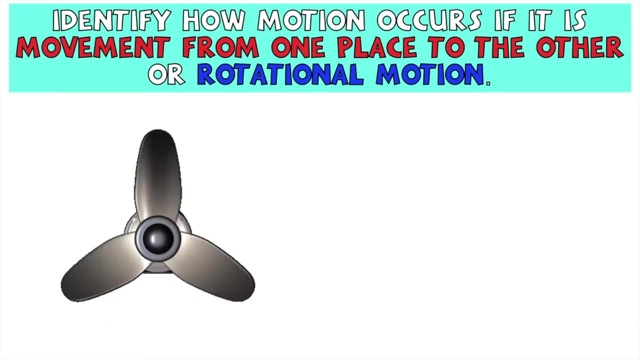 Is it movement from one place to the other or rotational motion? That's correct, children. The answer is movement from one place to the other. How about this one? That's correct. That's correct. The answer is rotational motion. How about if you have this? 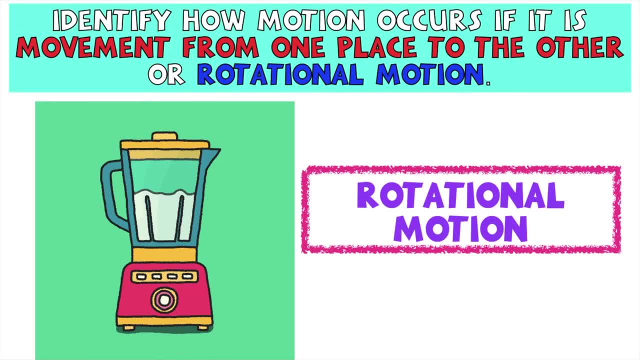 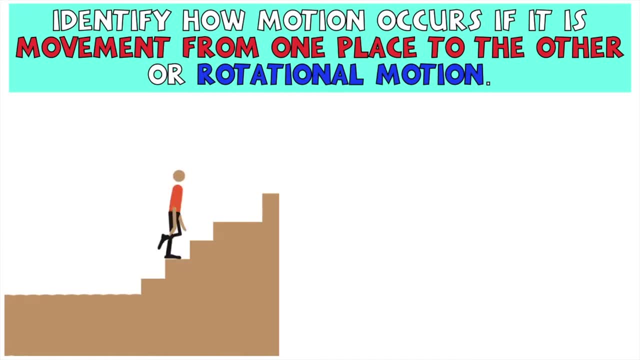 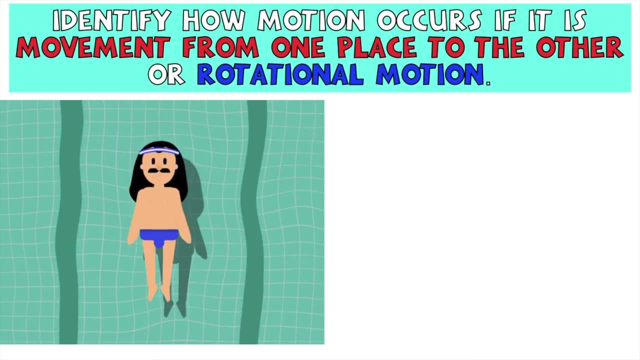 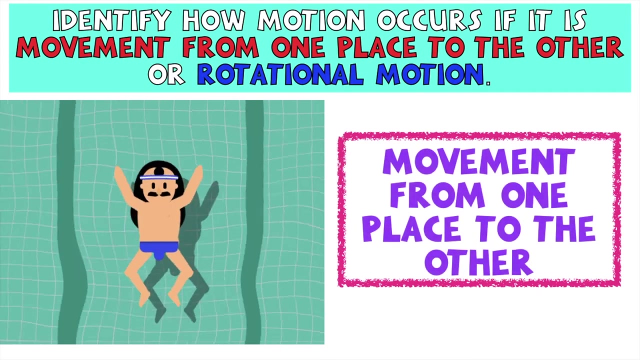 Very good, The answer is rotational motion. How about if you have this? Good job, children. This is movement from one place to the other. How about if you have this? Very good, The answer is movement from one place to the other. 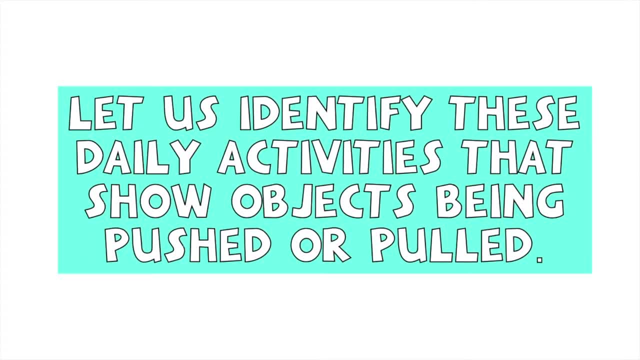 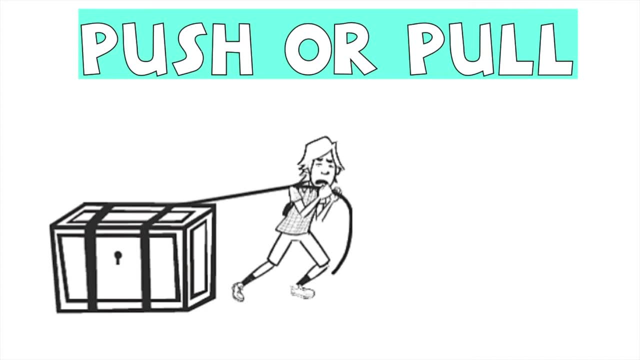 So now let us identify these daily activities that show objects being pushed or pulled. Let's have the first one. Is it push or pull? Very good, The answer is pull. How about if you have this? Is this push or pull? 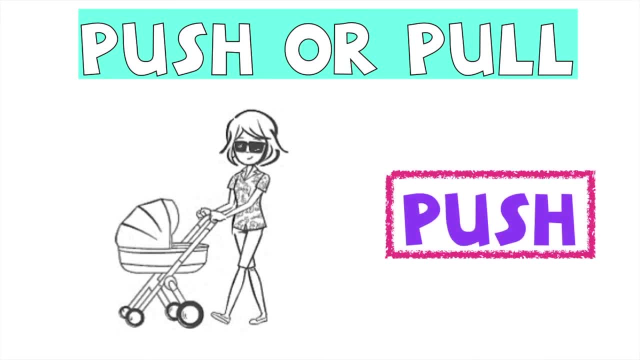 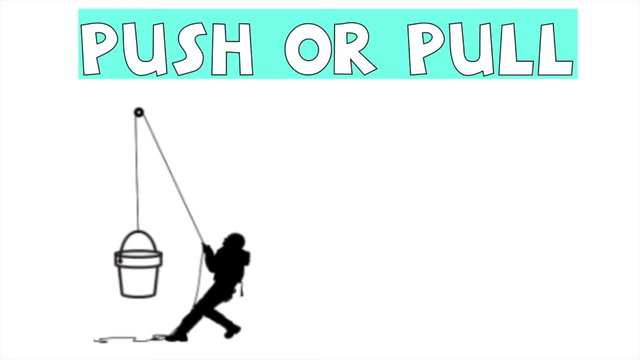 Good job, children, This is push. How about if you have this? Is this push or pull? Good job, This is pull. How about if you have this? Very good children, This is push. How about if you have this? 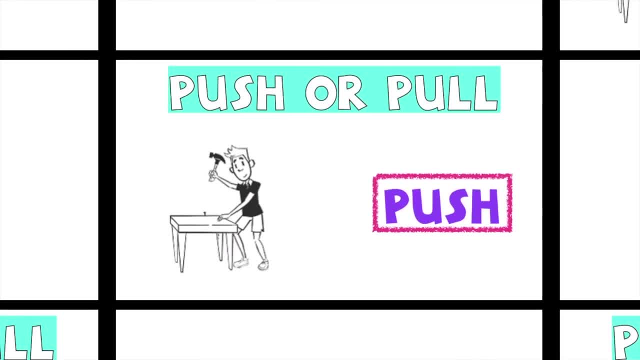 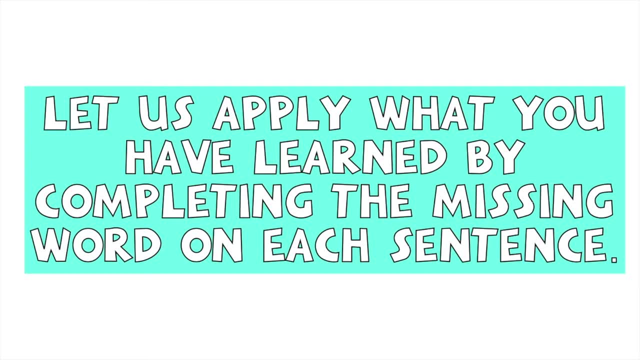 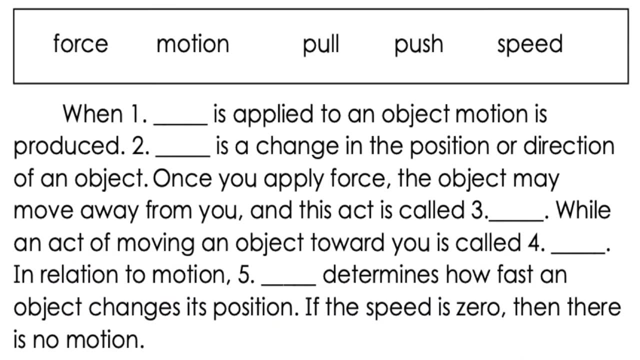 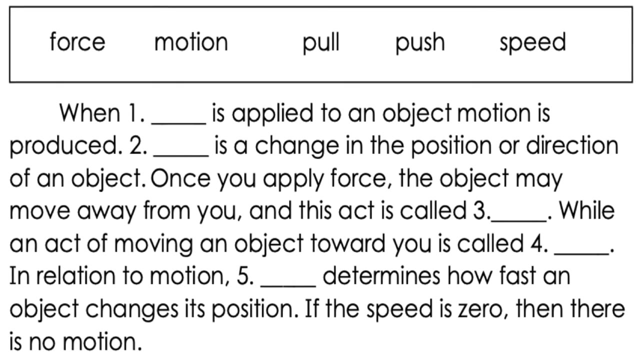 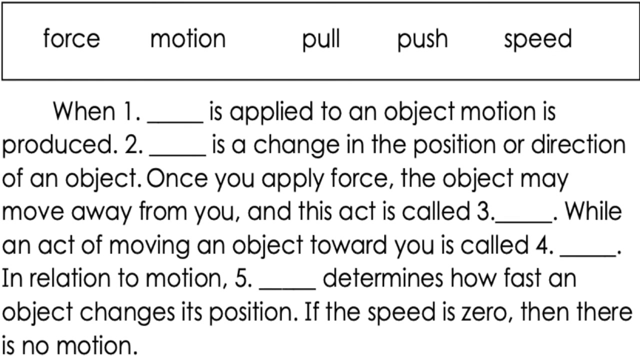 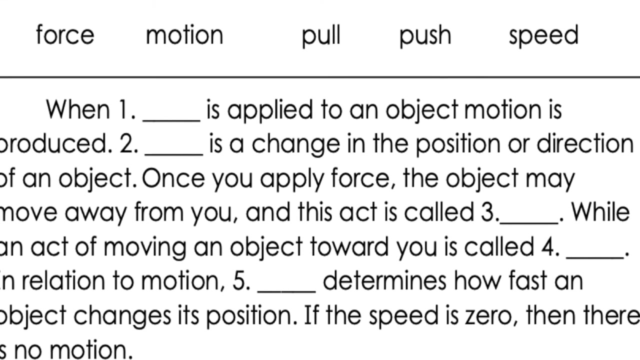 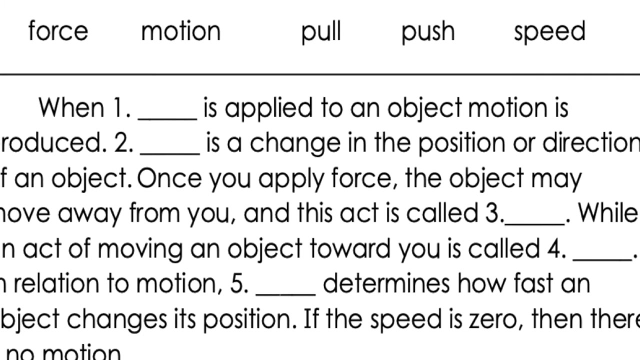 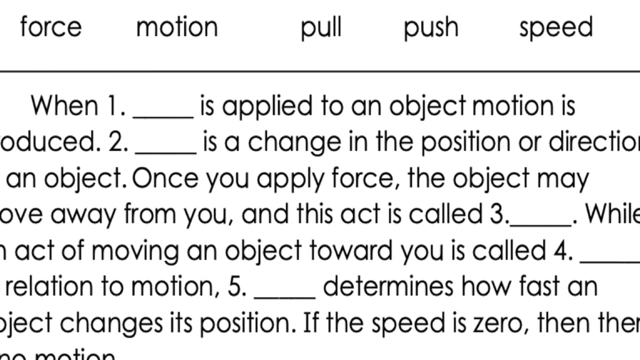 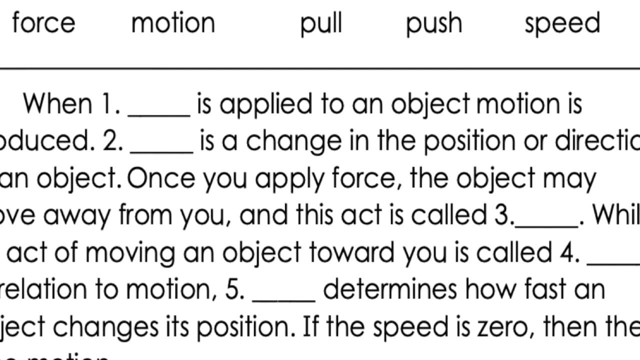 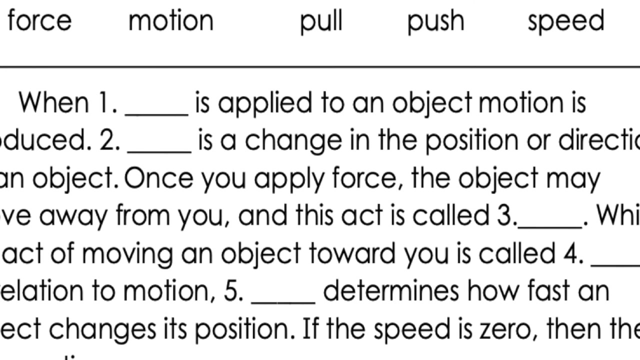 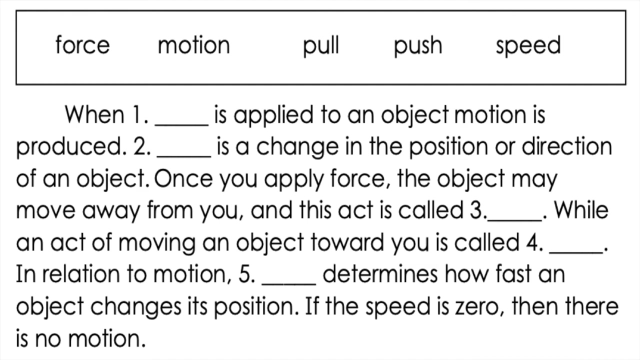 Your job. this is push. So now let us apply what you have learned by completing the missing word on each sentence. Are you ready? Are you ready? Are you ready? So, when blank is applied to an object, motion is produced, what is it?